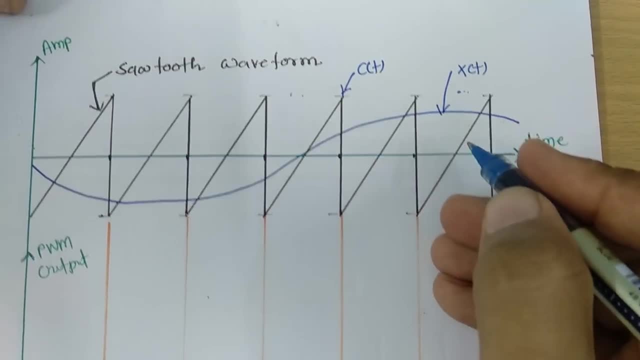 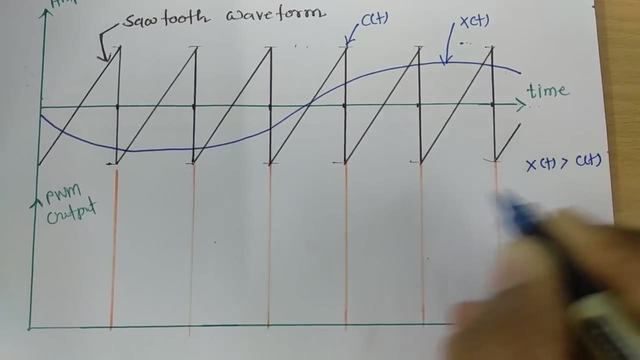 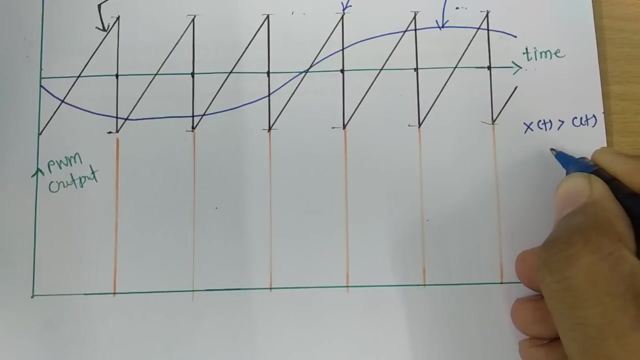 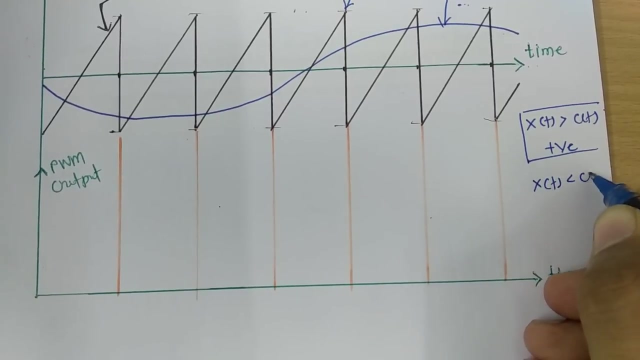 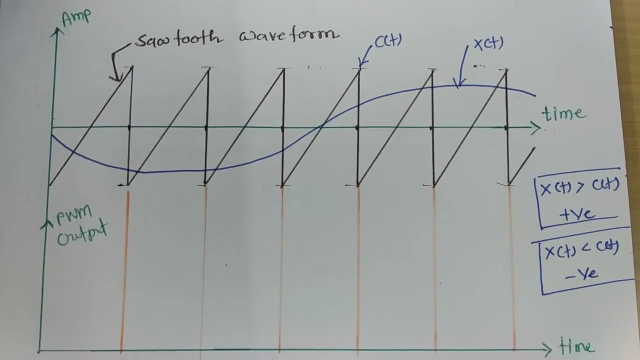 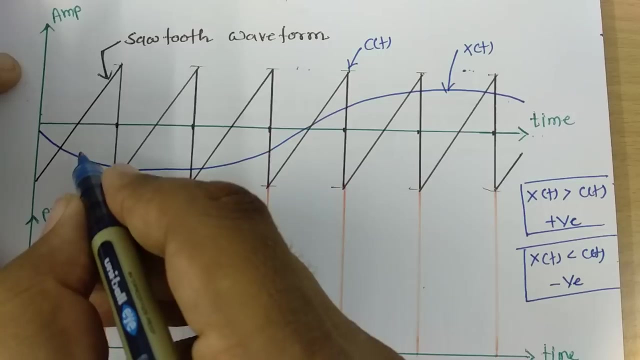 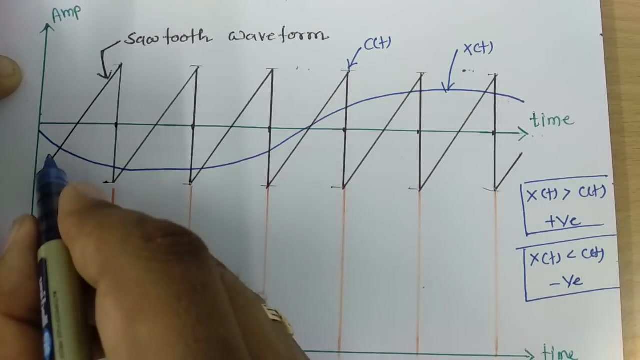 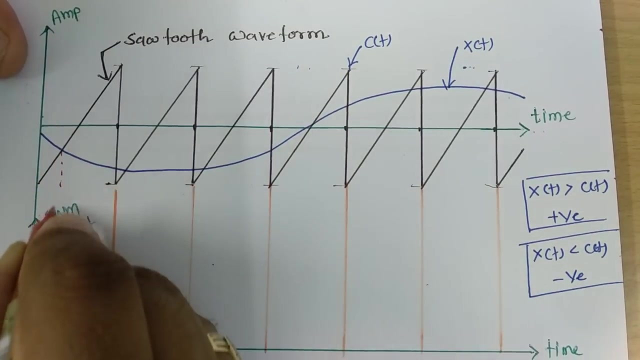 ct. Now I have already told like: see, if xt is greater than ct, output will be plus voltage. So in that case output will be positive voltage, and if xt that is less than ct, in that case output will be negative voltage. That is how this circuit functions. So let us try to make waveform out of this. So here one can clearly see: this is what xt right Now see. for this period xt is greater than this up to this point. So if I trace a trajectory, first of all let me trace out trajectory at this sample. See, I need to. 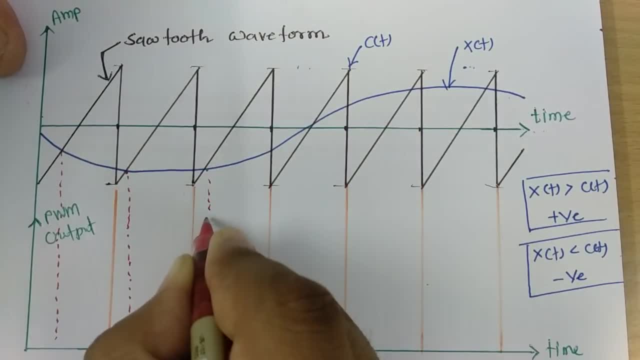 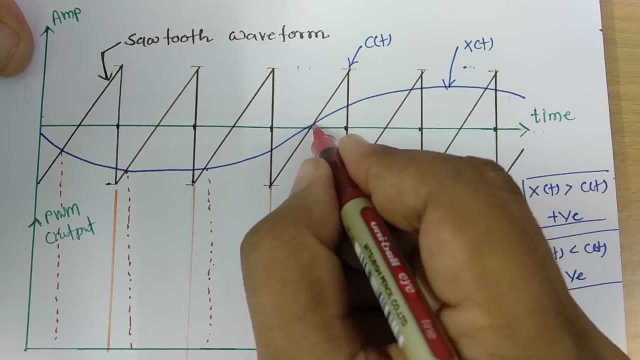 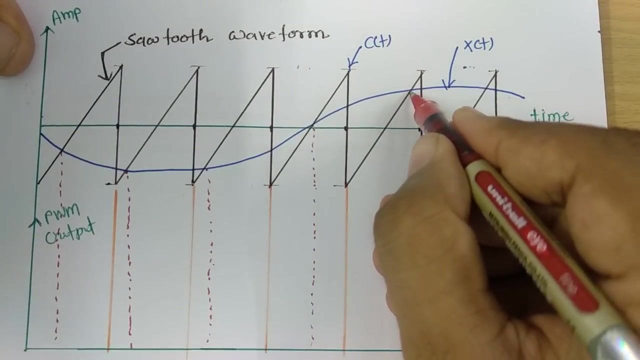 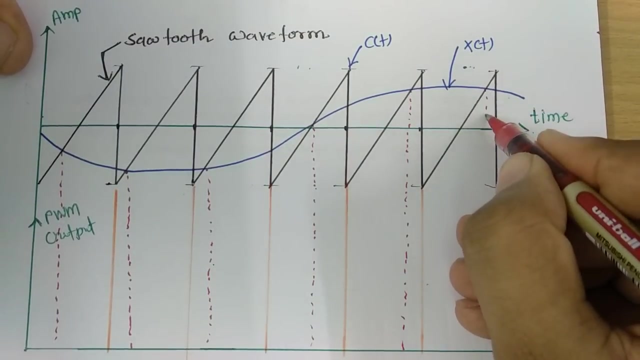 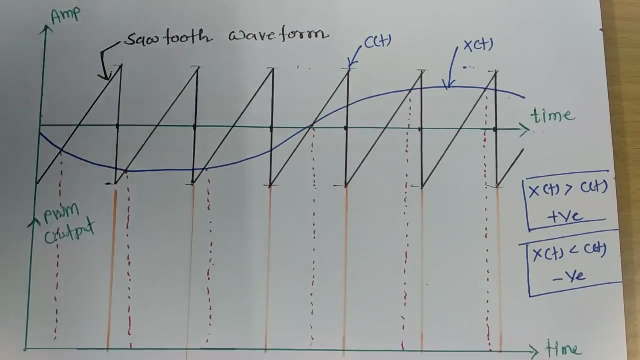 trace a trajectory. See, from this point I am just tracing trajectory. Now see, from here I need to trace trajectory, From here I need to trace trajectory, and from here I will have to trace trajectory. now see, as I have told, if xt is greater than ct, then output will be positive. so see for. 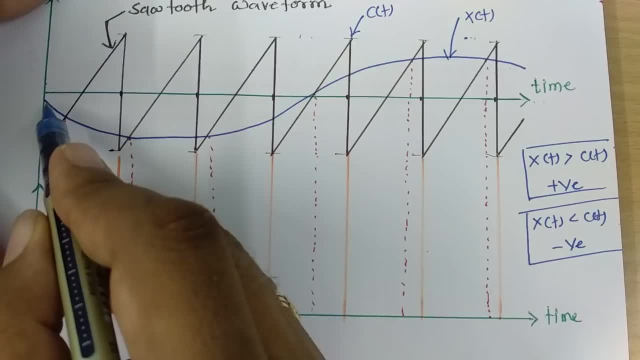 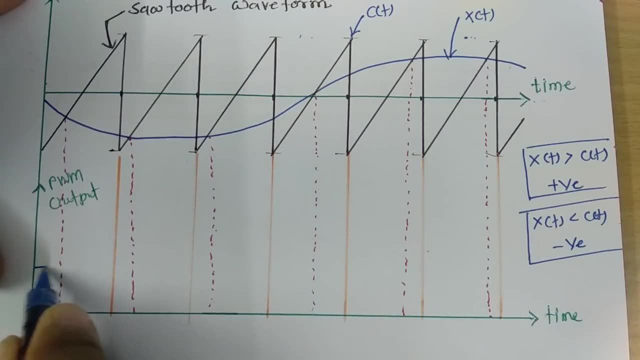 this interval, xt. that is this. by this blue color. it is greater than this. this is what black color. so there will be positive output. so you will be finding there will be positive output. and if ct is greater than xt, then there will be negative output. so you will be finding: 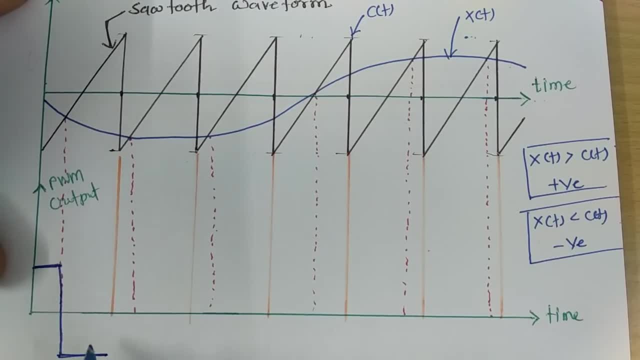 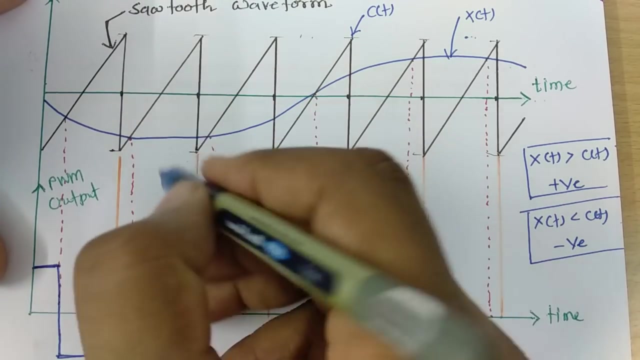 up to this, there will be negative output. now see for this region again: xt is greater than ct, so there will be positive output. and in this region, ct is greater than xt. you can see this is ct, that is greater than xt, so there will be negative output. so see this. 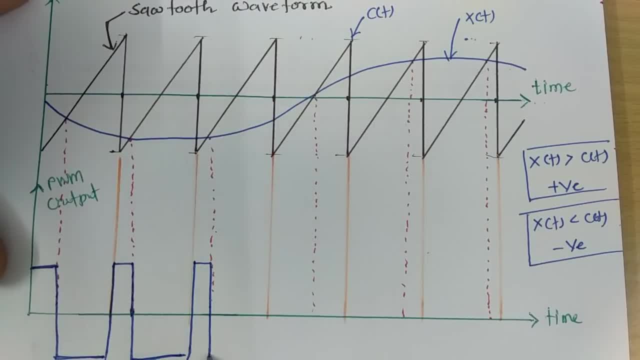 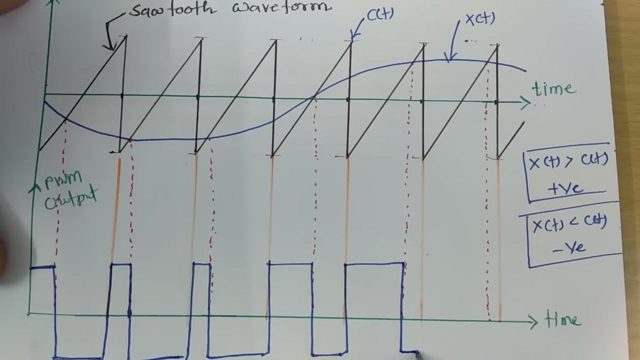 is what keeps on repeating and you will be finding waveform that is pulse width modulation, modulated waveform. so this is what the output, as if xt is greater than ct, there will be positive output. if xt is less than ct, there will be negative output. and this is how waveforms. 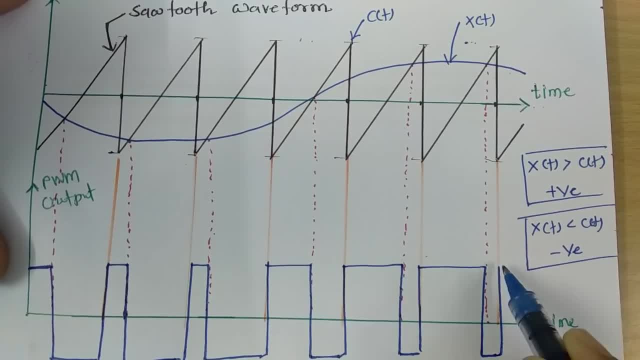 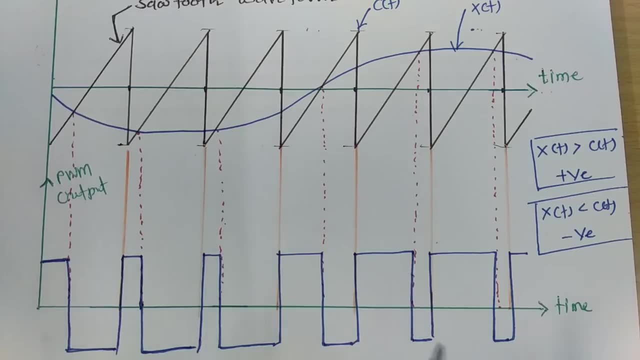 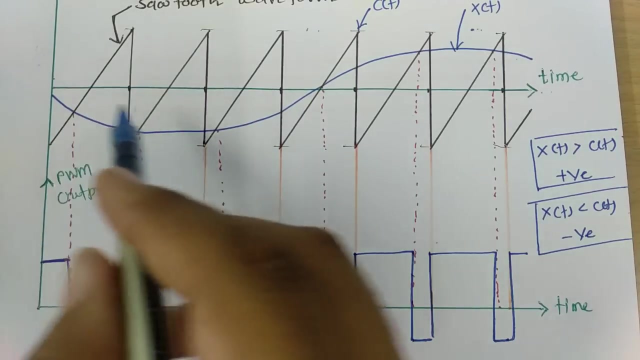 are coming. so you will be finding this is what pulse width modulated output. this is PWM output, where here you will be finding positive width is more, and over here you will be finding negative width is more. So that shows like see, what is modulating signal. so this is what all about PWM output. 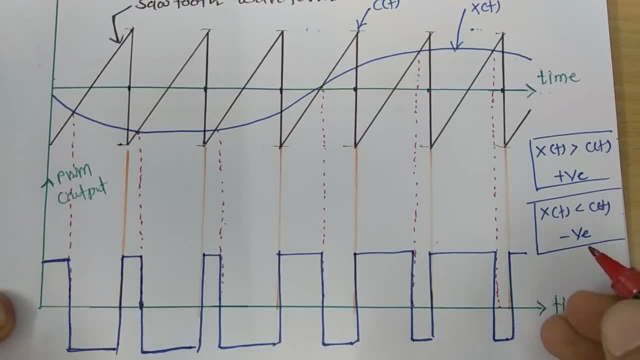 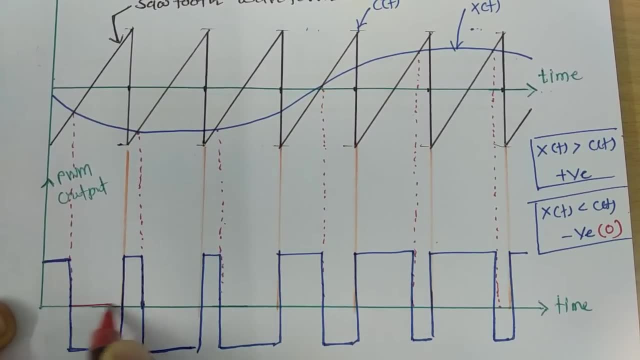 in some cases you will be finding it is given with respect to reference. so if I say if xt is less than ct, then if my output is 0, so in that case your waveform will be this: instead of negative, you will be getting 0 voltage. so see, this is what even you can do, like in. 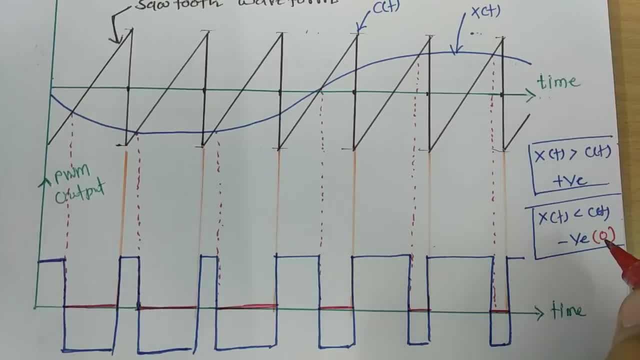 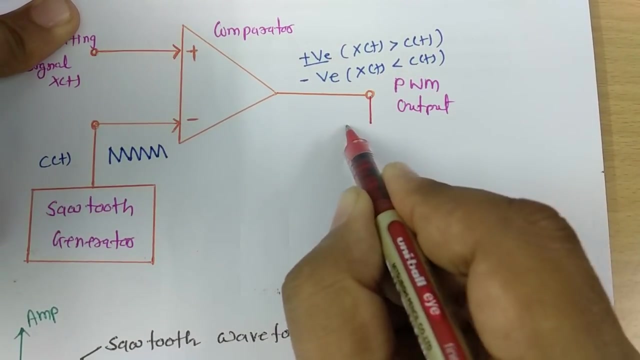 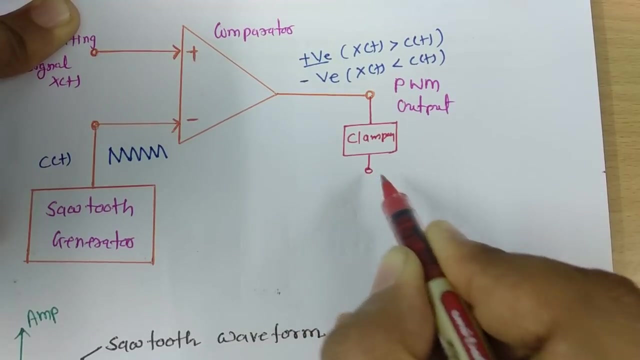 operation If xt is less than ct, in that case there will be negative output that we can have so that even possible by adding one more additional circuit by using clamp clamper over here- if I use clamper circuit, So over here we will be having PWM output. 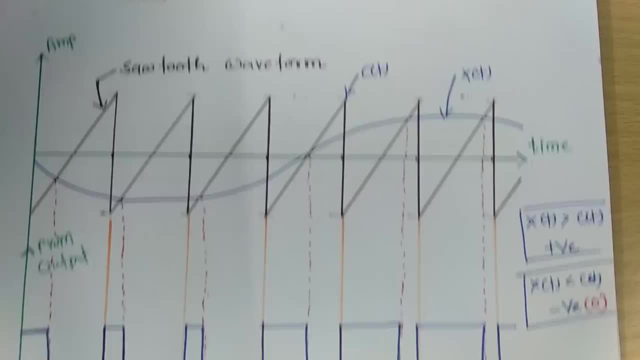 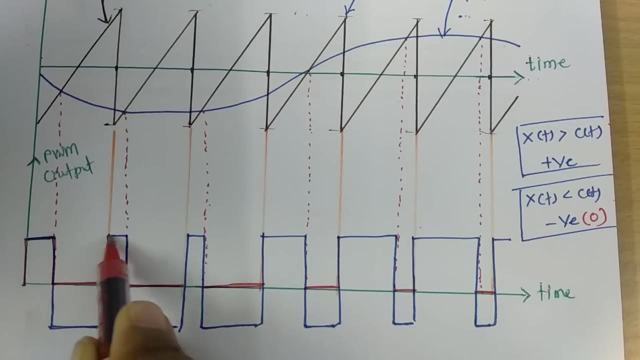 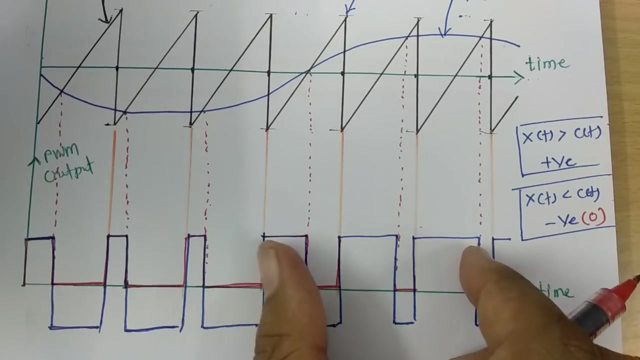 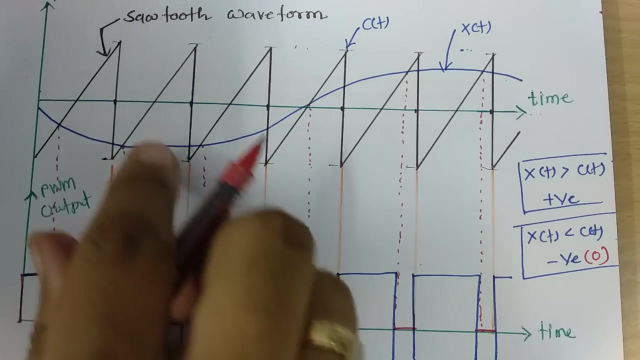 But in this PWM output your output will be there with respect to zero voltage, so actual waveform will be this. so in that case you will be finding actual voltage signal. that will be this where you will be finding: over here output. voltage is high. the reason is amplitude is positively high and over here output is low. the reason is modulating signal. 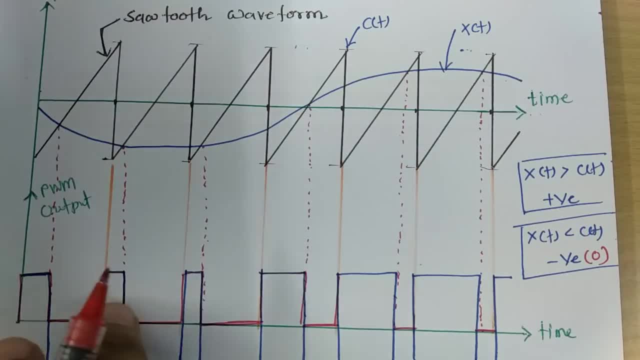 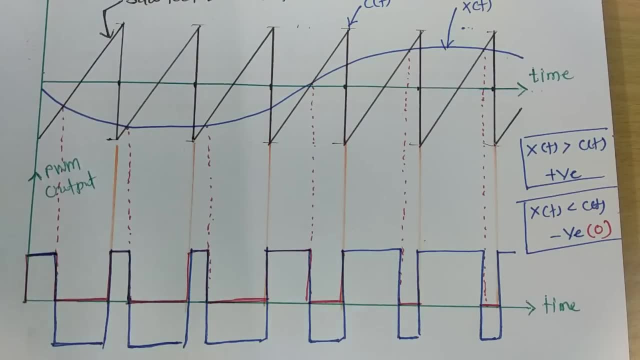 is negative over here. So here, with respect to input signal, we will be generating PWM output. that is this. So this is about pulse width modulation and that is how we can generate it. Thank you so much for watching this video. In next session, I will explain you pulse position modulation, PPM. so just stay tuned with this.